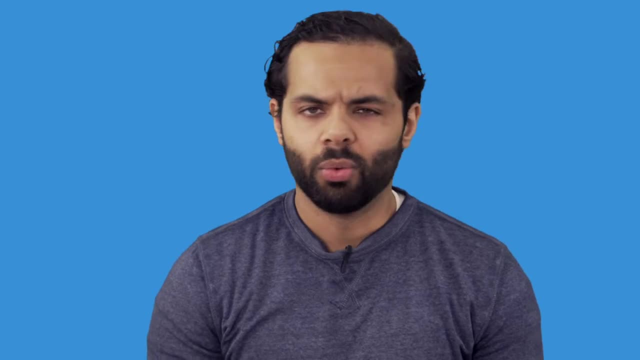 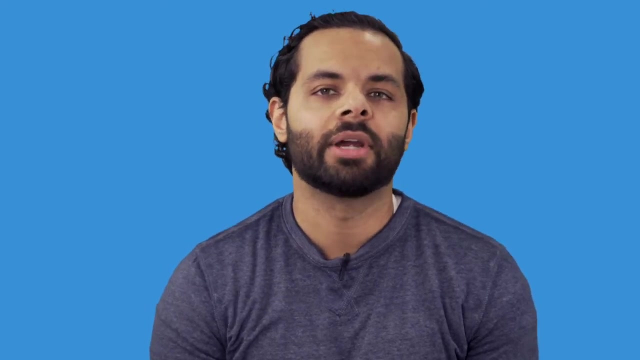 If you've stumbled upon this video, then you're probably asking yourself: what is Calculus AB versus Calculus BC, Or which one should you take? These are questions that many students and parents have when preparing their high school and college schedules. so you're not alone. 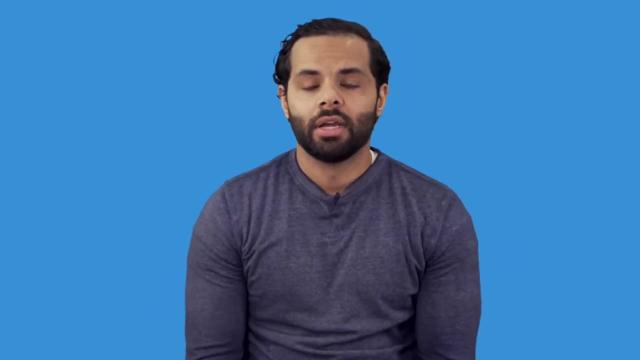 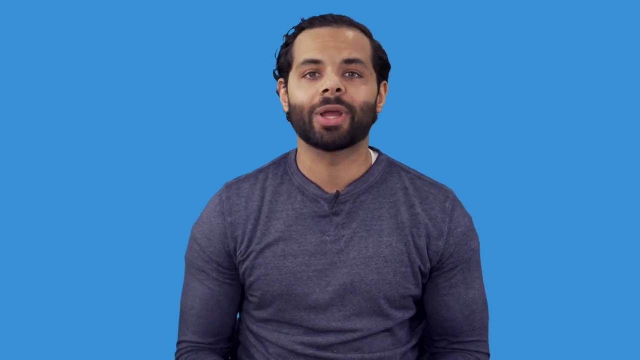 Figuring out the answer requires you to learn. I'm going to talk about what both courses offer, their exam setups, and weigh this information against your credit requirements and academic and personal goals. So I'll start by looking at the general overview of Calculus and then the Calculus AB and BC options individually. 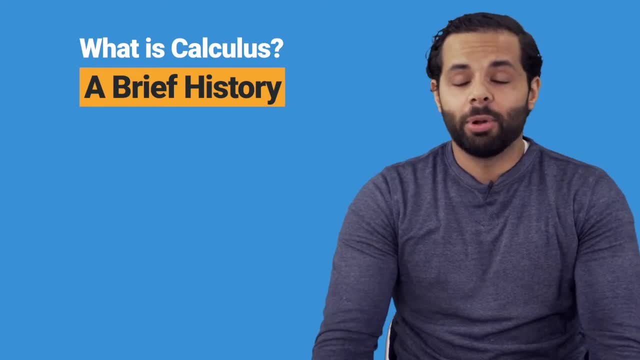 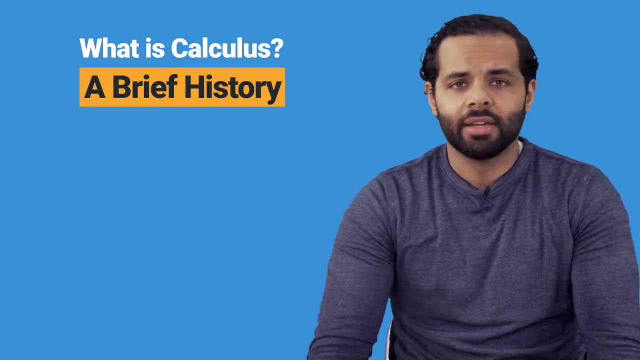 So first up, what is Calculus? A brief history. If you polled 100 people on the street and asked them the question, what is Calculus, the majority would answer something along the lines of hard math. It's not until a person is faced with the task of choosing between math courses. 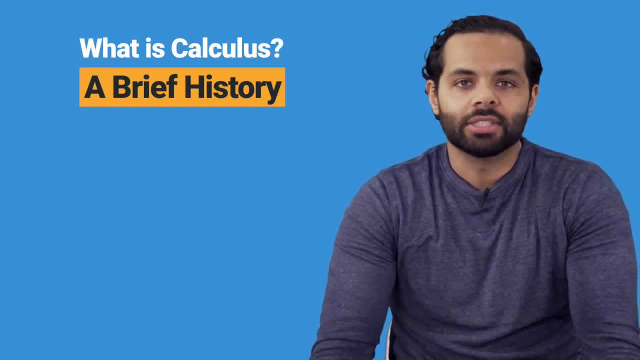 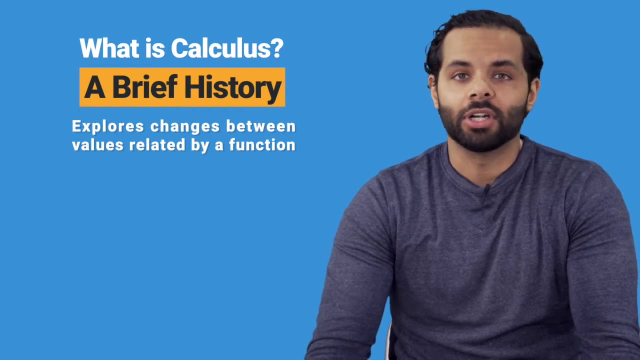 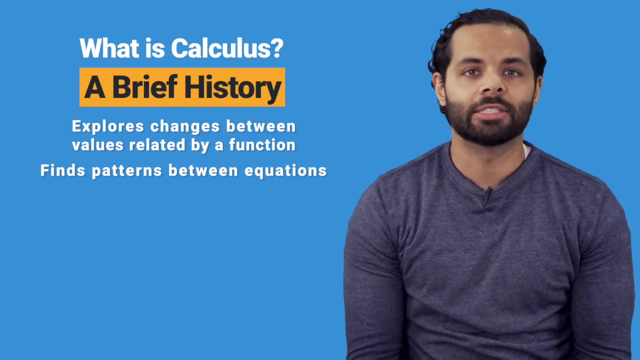 does one actually consider what these courses are made of? Calculus is a problem-solving branch of mathematics that does the following: It explores changes between values related by a function. It finds patterns between equations. Both Isaac Newton and Gottfried Willeblibnes independently discovered the concepts that make up calculus in the 1600s. 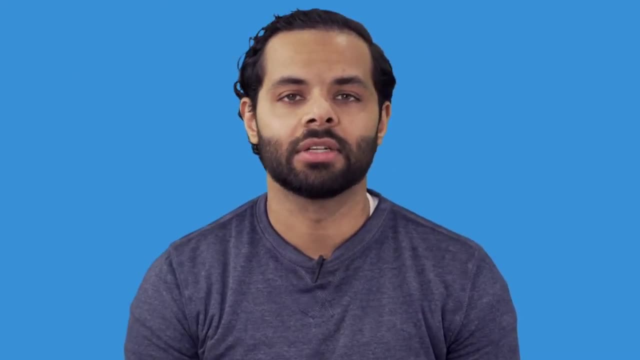 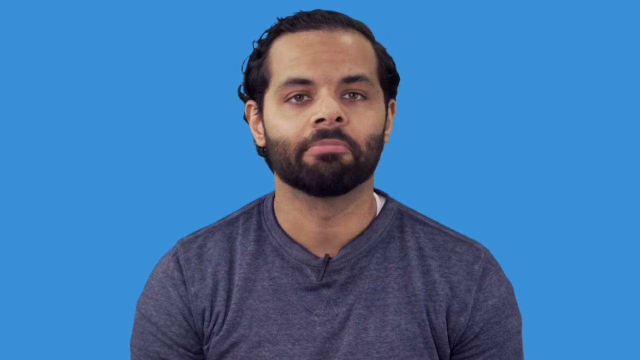 People have been using it to create mathematical models ever since The discipline grew out of the desire to understand natural phenomena such as orbiting planets and gravity in a deeper way. This explains why so many science-based fields require an understanding of calculus. 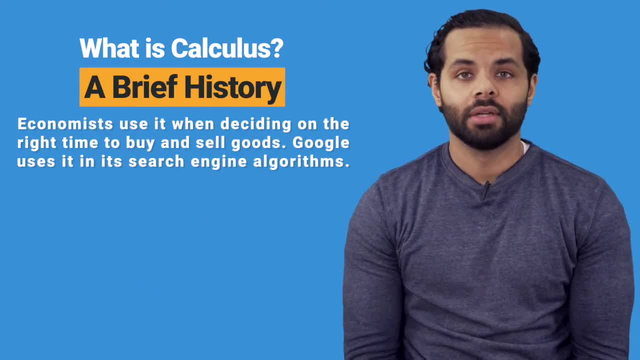 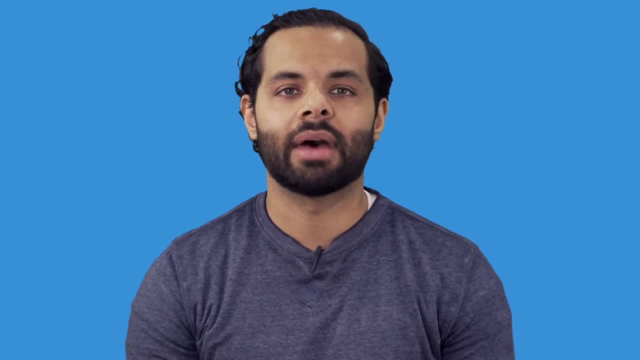 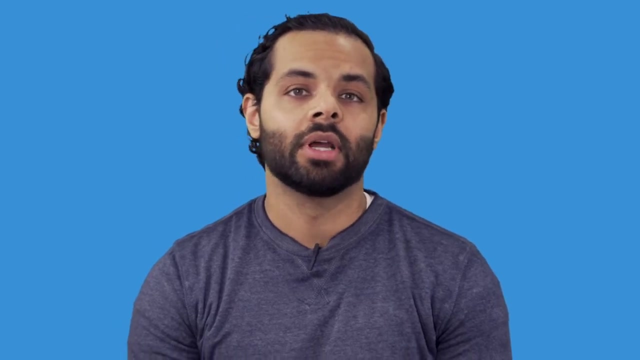 Economists use it when deciding on the right time to buy and sell goods. Google uses it in their search engine algorithms. The field of engineering in particular requires its specialists to understand the mathematical study of change. Many engineers use calculus in their everyday designs, using it to decide on the size and shapes of curves when building structures. 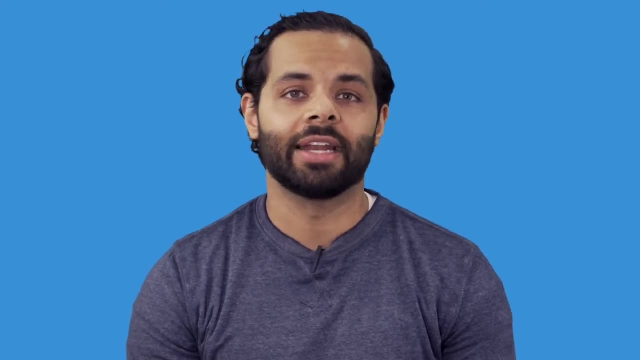 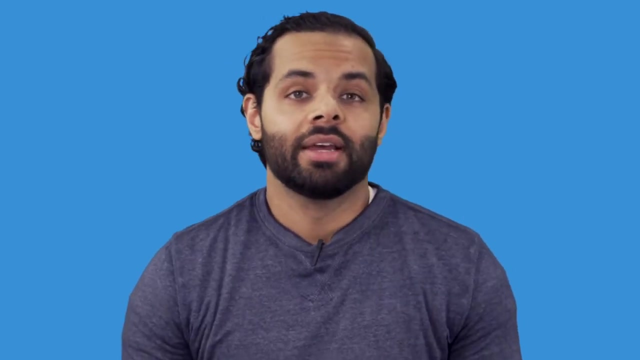 Although it's a dreaded subject by some, calculus is very useful, as it can help you solve problems in many other fields, including engineering, physics, economics, biology and medicine. So, who knows, maybe this can be one of the easier courses you take. 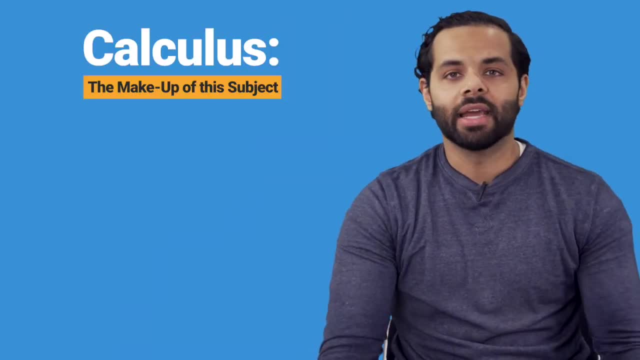 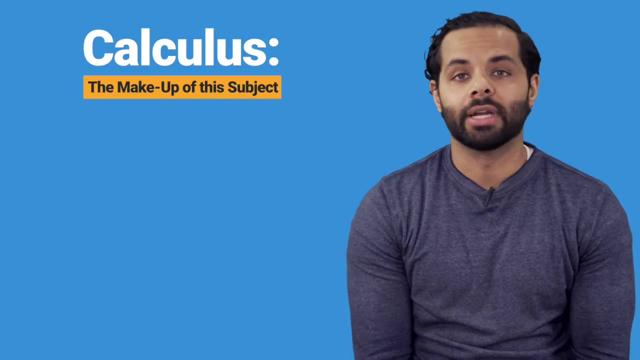 Next up is calculus- the makeup of the subject. Before taking calc, most students are required to complete four years of secondary math, like algebra 1, algebra 2, geometry and trigonometry. Pre-calc is usually a requirement, especially at the college level. 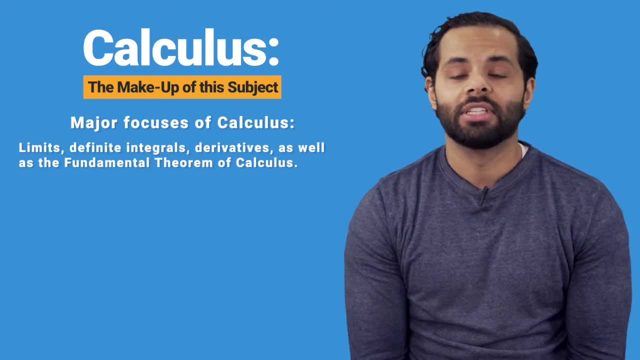 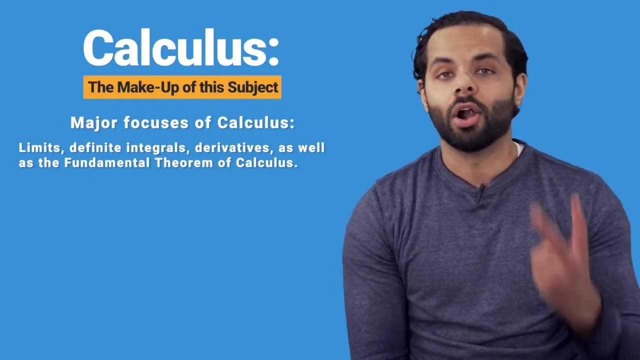 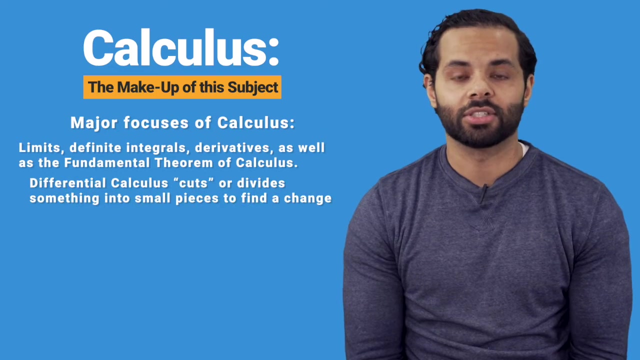 Major focuses of calculus include limits, definite integrals, derivatives, as well as a fundamental theorem of calculus, Which leads to an important point. There are two different types of calculus: differential calculus and integral calculus. Integral calculus cuts or divides something into small pieces to find a change. 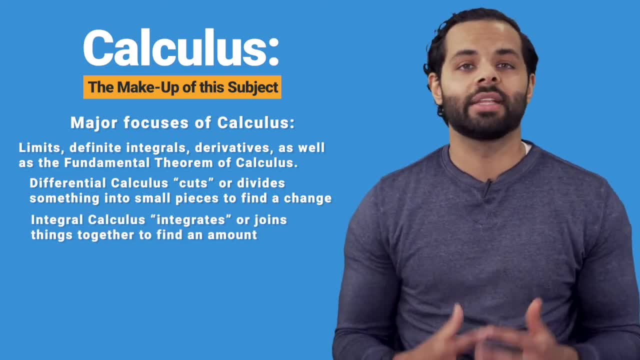 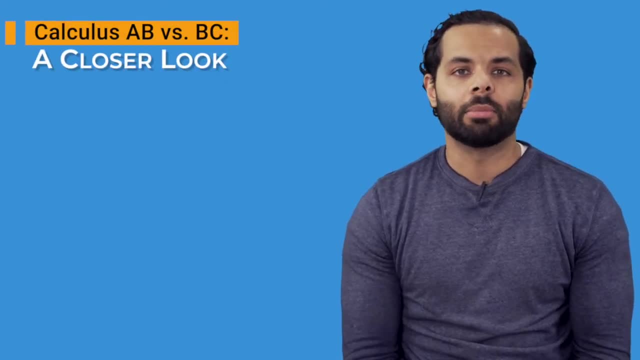 Integral calculus integrates or joins things together to find an amount Alright. so let's move on to calculus AB vs BC a closer look. The main thing to remember about the difference between BC and AB is this: Calculus BC is a review and continuation of calculus. 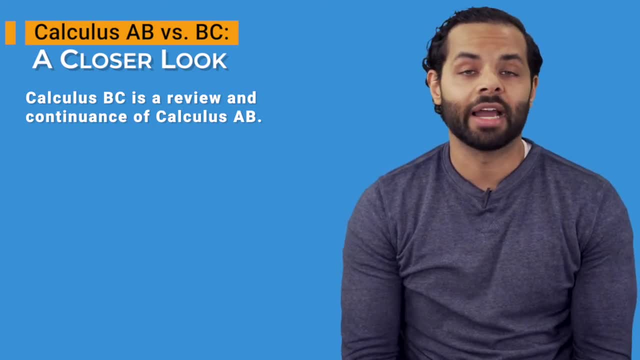 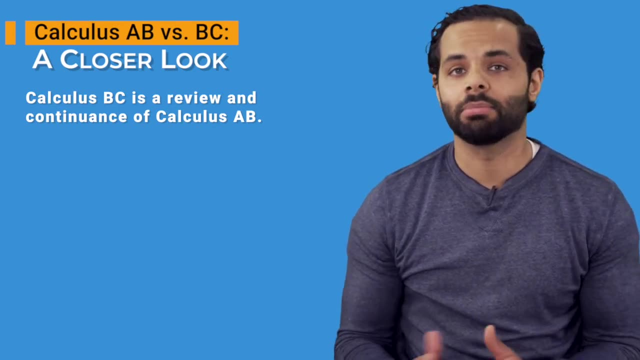 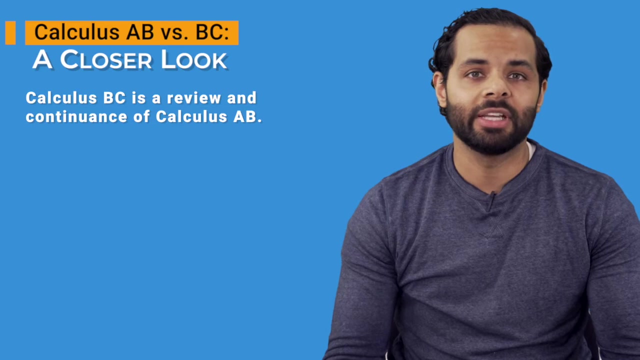 BC can be viewed as an offshoot of calculus AB, since all the topics in calculus AB, which is single-valuable calculus, are also included in calculus BC, plus some more. Unlike courses like algebra 1 and algebra 2,, calculus AB, advanced placement calculus and calculus BC do not have to be taken in a specific sequence. 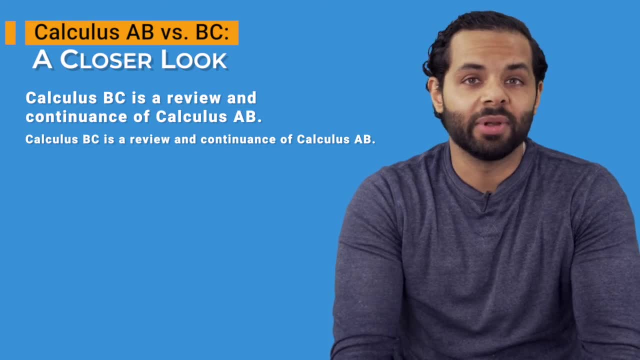 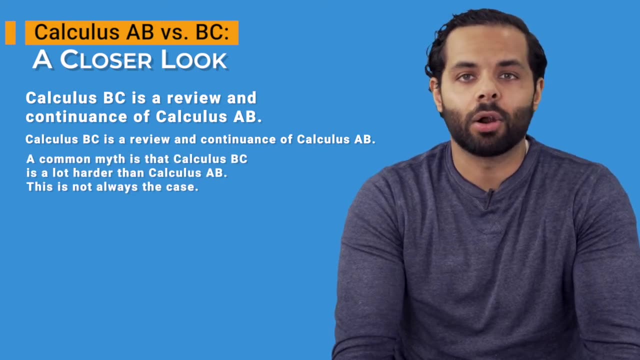 Keep that in mind. This means that you could take calculus BC without having ever taken calculus AB. Many students do this. A common myth is that calculus BC does not have to be taken in a specific sequence. Calculus BC is a lot harder than calculus AB. 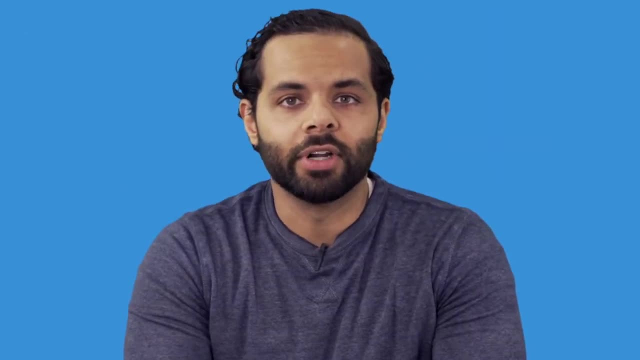 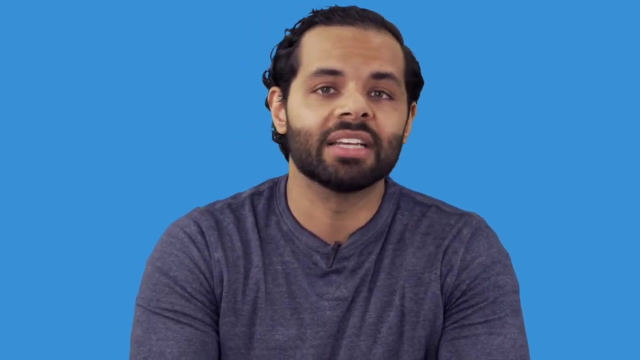 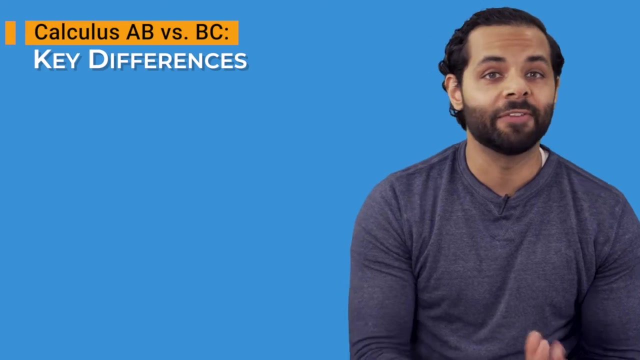 This is not always the case. These two calculus courses are different in scope but not necessarily in complexity. Calculus BC is only considered a more difficult course by some because it covers more material. Calculus AB vs BC: the key differences: Here are some fundamental similarities and differences between the two. 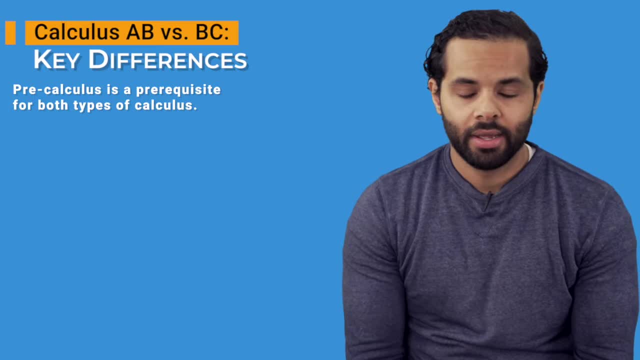 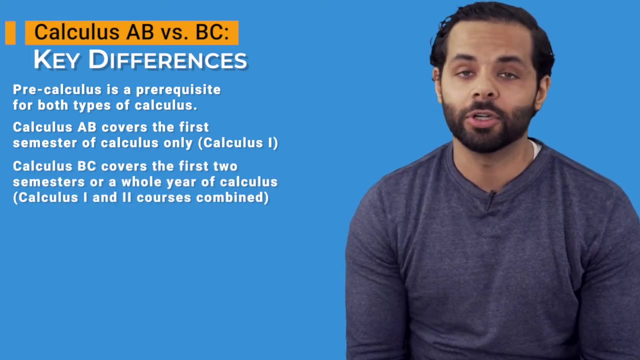 Pre-calc is a prerequisite for both types of calculus. Calculus AB covers the first semester of calculus only, which is calculus 1.. Calculus BC covers the first two semesters or a whole year of calculus, which is calculus 1 and 2 courses combined. 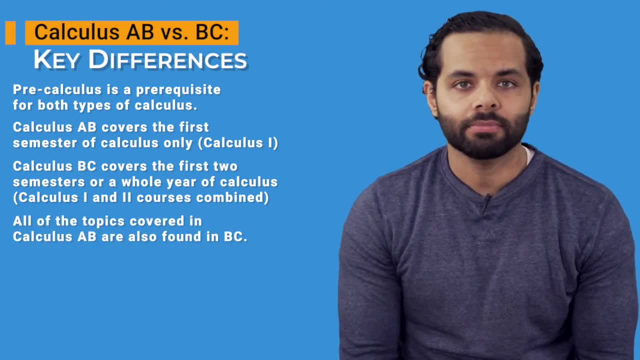 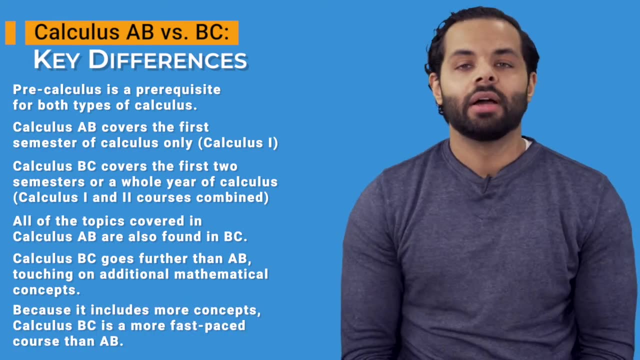 All the topics covered in calculus AB are also found in BC. Calc BC goes further than AB, touching on additional mathematical concepts. Because it includes more concepts, calculus BC is a more fast-paced course than AB. Let's move on to calc AB vs BC: scope and sequence. 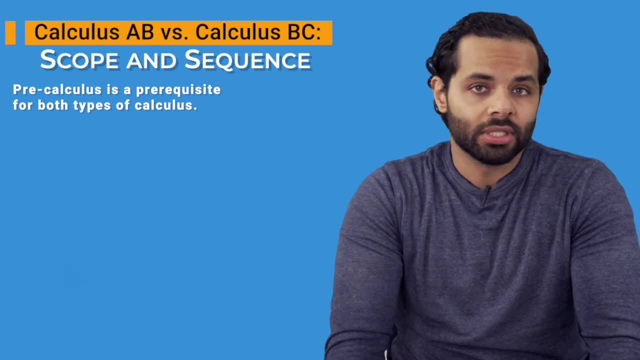 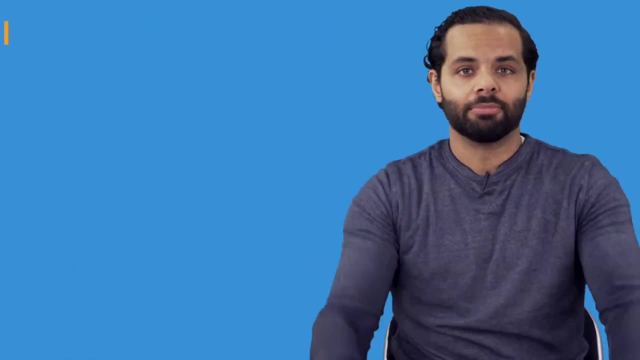 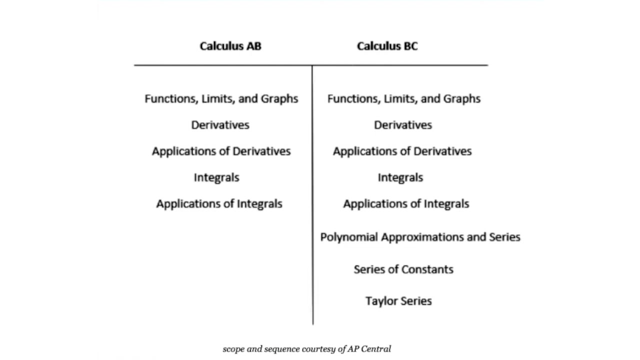 Although the sequence of the topics can vary by school and course, the T chart that I'm going to provide you in just a second provides a general comparison of the two different tracks. Here you go. As you can see, calc BC is not a different course from calc AB. 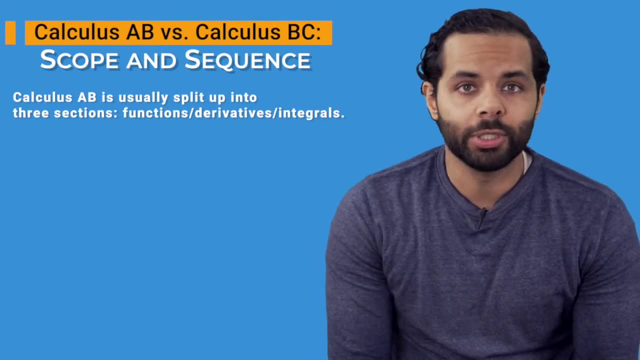 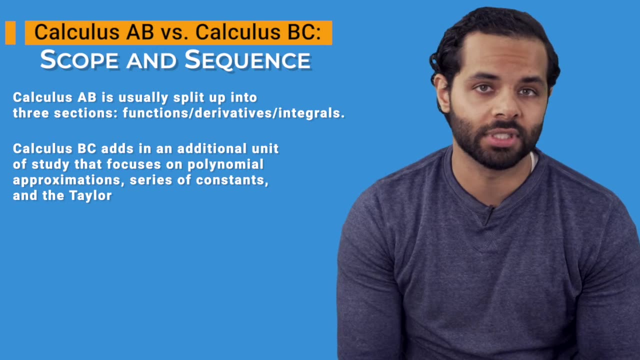 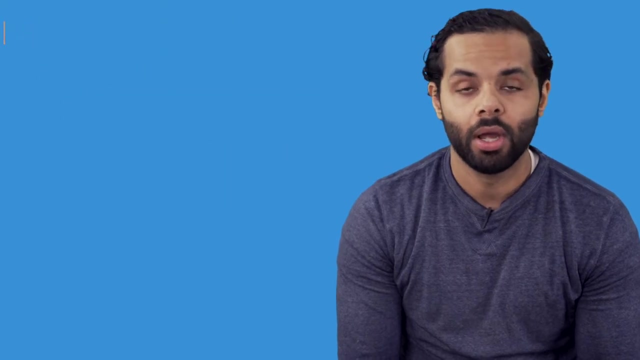 It is a more in-depth version. Calc AB is usually split up into three sections: functions, derivatives and integrals. Calc BC adds an additional unit of study that focuses on polynomial approximations, series of constants and the Taylor Calculus. AB and BC exam overview. 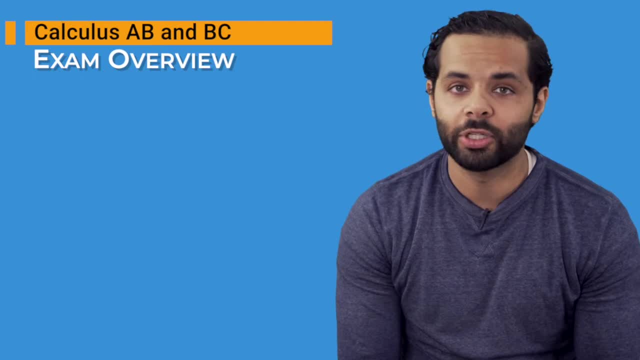 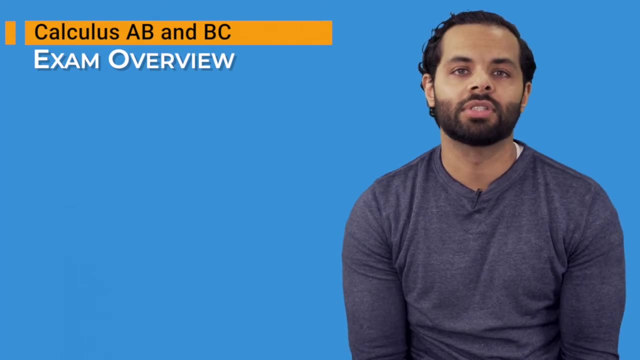 When deciding on which type of calculus to take, it can be beneficial to take a more in-depth look at what is included on the exam for each course. This will allow you to decide if you're ready to take on either course of study or maybe even both. 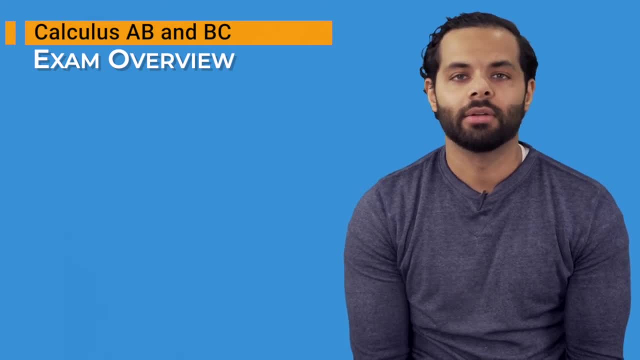 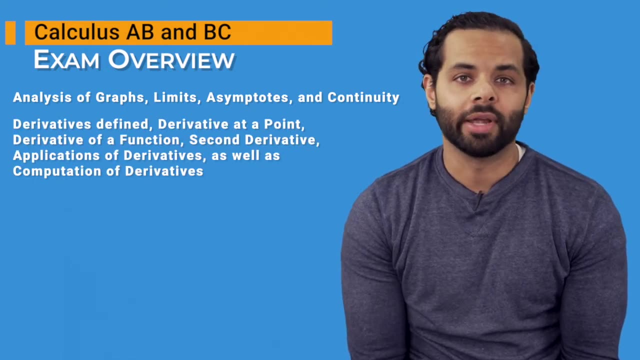 According to the Princeton Review, AB typically includes the following: Analysis of graphs, limits, asymptotes and continuity. Derivatives defined Derivative at a point. Derivative of a function, Second derivative. Applications of derivatives, as well as computation of derivatives. 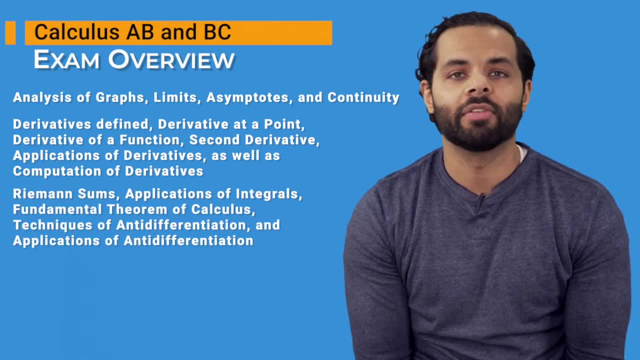 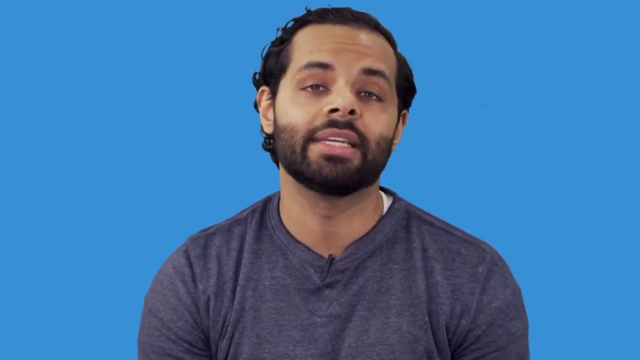 Riemann sums: Applications of integrals, fundamental theorem of calculus, techniques of anti-differentiation and applications of anti-differentiation. All these topics will be on the BC exam as well. The test will also cover polar and parametric functions. 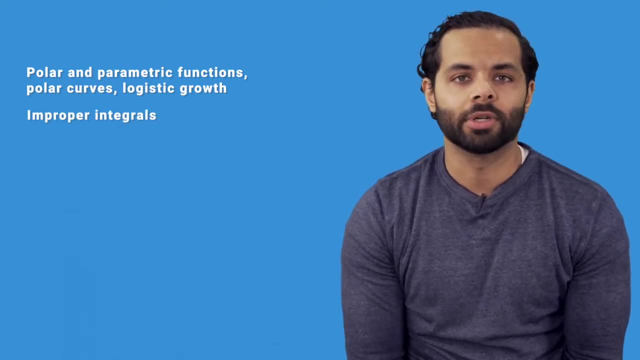 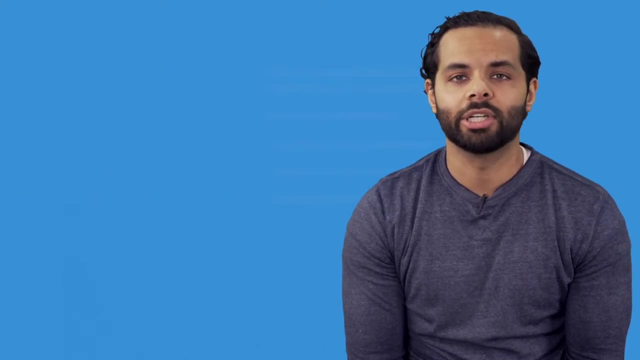 polar curves, logistic growth, improper integrals, Taylor series and powers, radius and interval of convergence, Taylor polynomials and approximation. Many of the same topics found on the Calculus AB exam will also appear on a test assessing the understanding of Calculus AB. 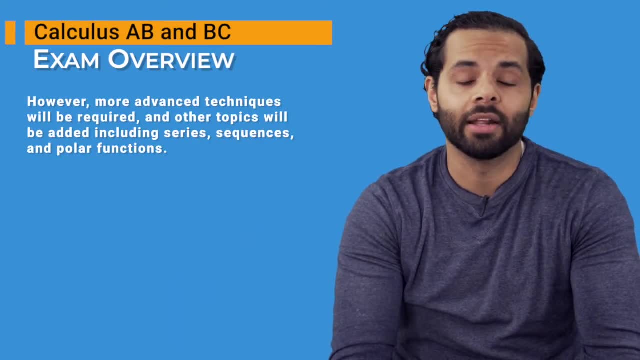 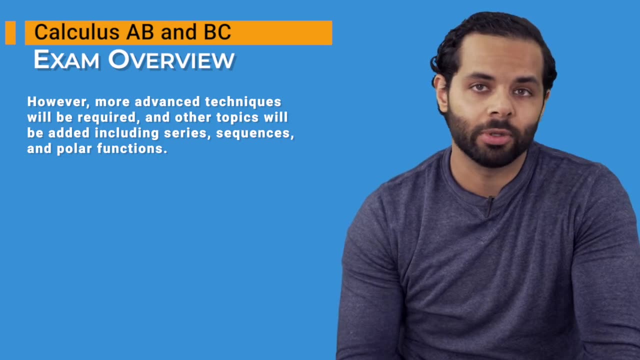 However, more advanced techniques will be required and other topics will be added, including series, sequences and polar functions. When it comes to AP exams for college credit, the College Board schedules both the Calculus AB exam and the Calculus BC exam at the same exact time. 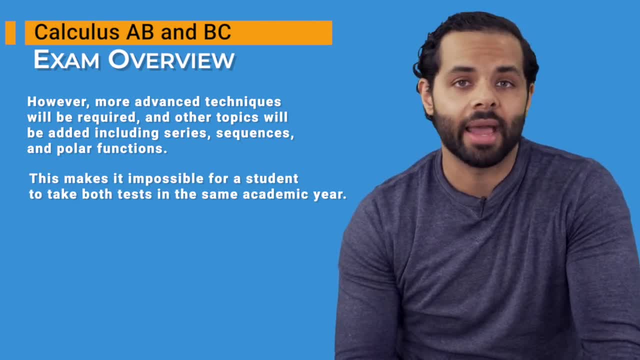 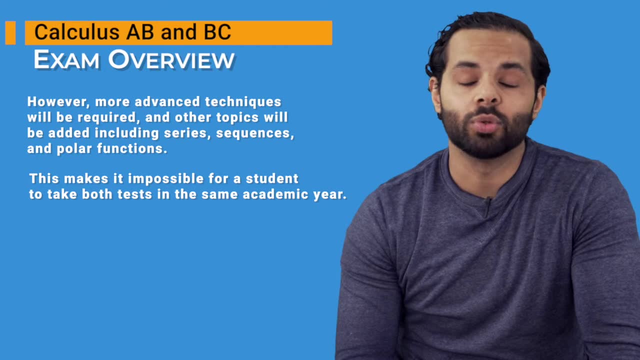 This makes it impossible for a student to take both tests in the same academic year. The exam structures are identical, as is the amount of time you get on the test. The main difference is what is included. Here's a table that breaks it all down for you. 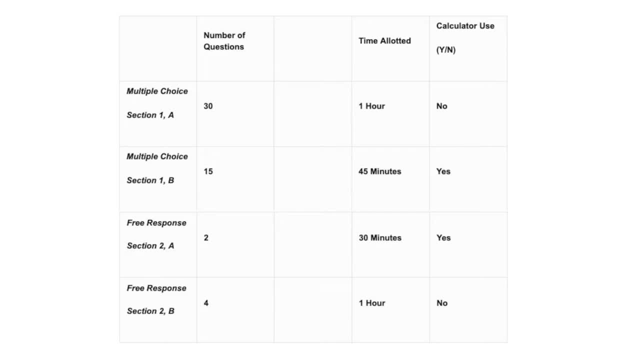 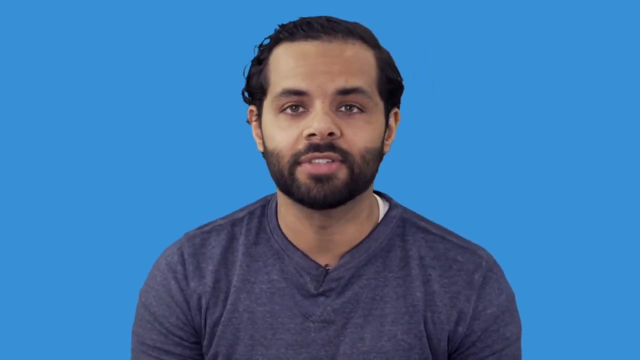 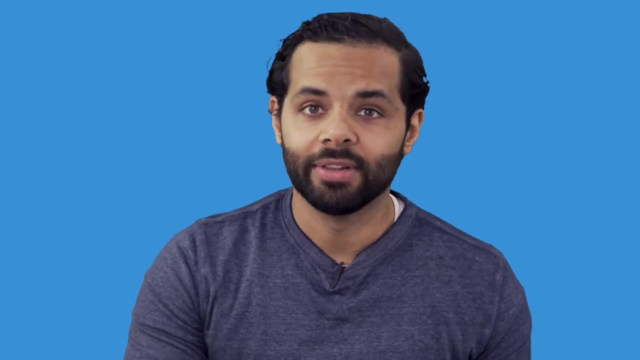 Enjoy. So now, this isn't to say that the BC test is harder. In fact, many students find Calculus BC's exam to be less challenging because of the way the material is distributed: Because there are more topics to cover, the questions are not heavily focused on any one particular area. 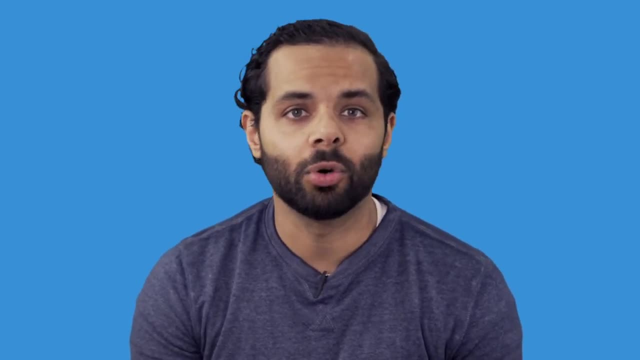 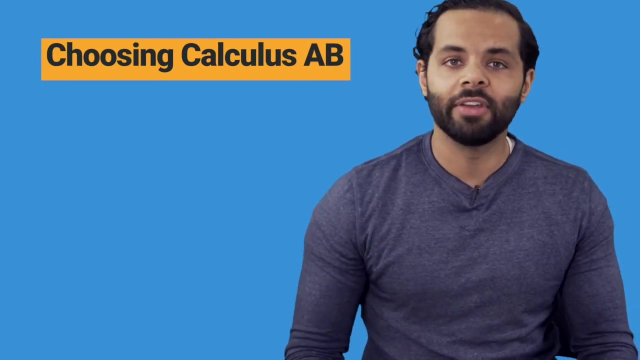 This allows for more breathing room, so to speak. if you struggle with a particular concept, Choosing Calculus AB, Now that you understand the difference between the two courses, you may be trying to figure out which to take. There is no right or wrong answer here. 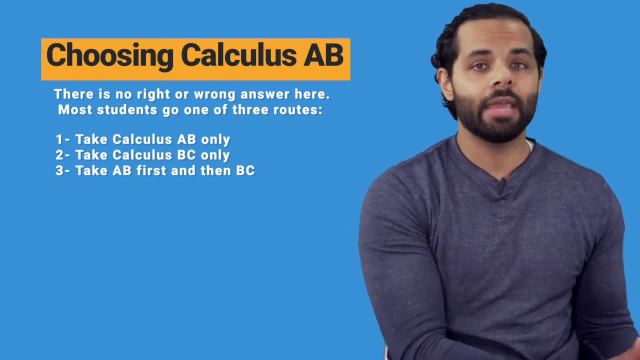 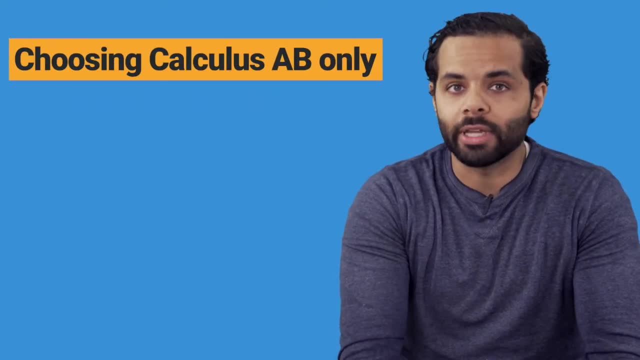 Most students go one of three routes: Taking AB only, taking BC only and then taking AB first and then BC afterward, Choosing Calculus AB only. Although you will get more college credit for taking Calc BC, it is not always the right option. 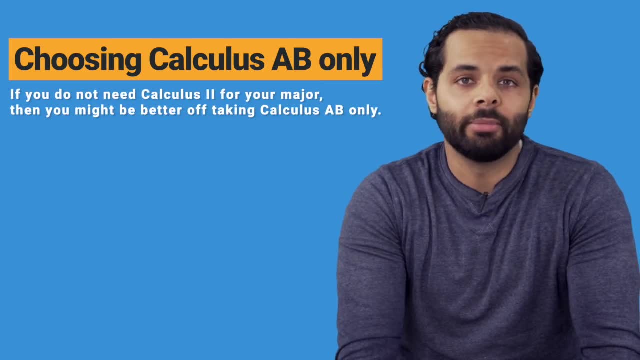 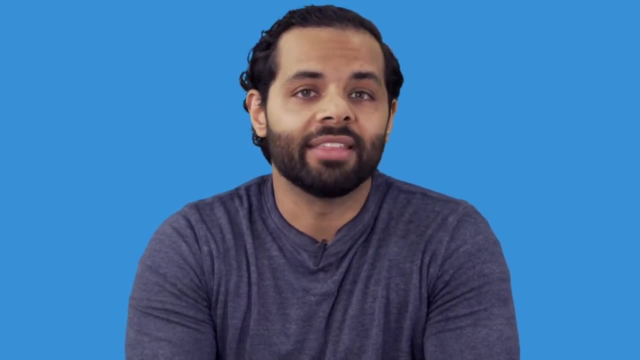 It's all subjective. If you do not need Calculus 2 for your major, then you might be better off taking Calculus AB only. The same can be said for students who struggle with math and think that a fast-paced course like Calculus BC 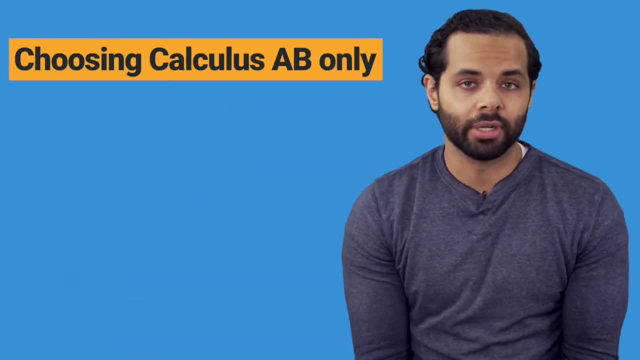 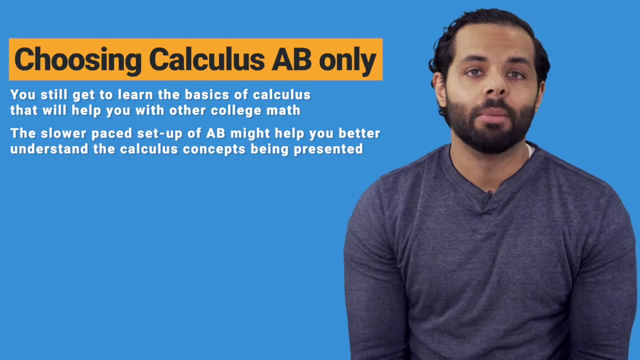 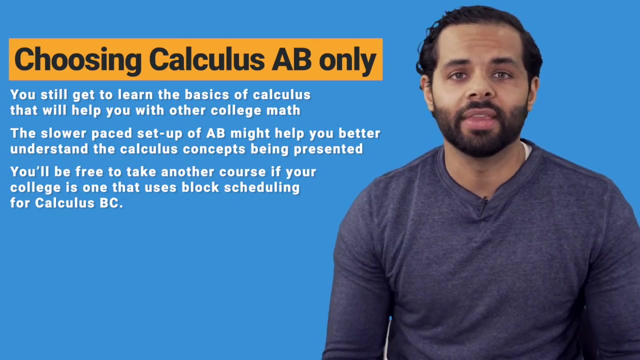 will be too challenging for them. Benefits of choosing this option include: you still get to learn the basics of Calc. that will help you with other college math. The slower-paced setup of AB might help you better understand the Calc concepts being presented. You'll be free to take another course if your college is one. 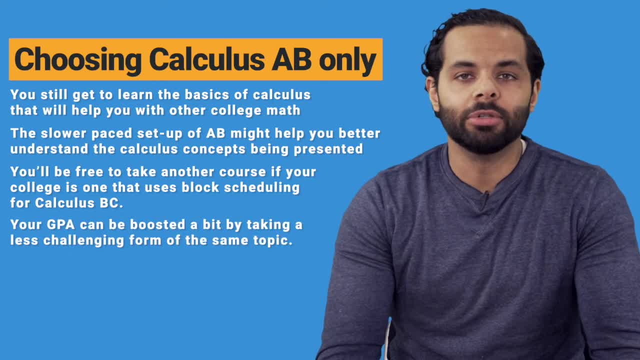 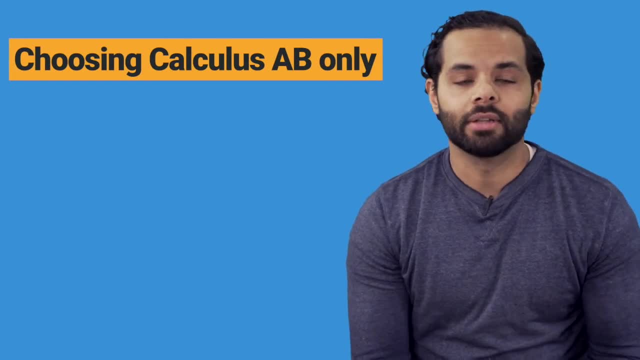 that uses block scheduling for Calc BC. Your GPA can be boosted a bit by taking a less challenging form of the same topic, Choosing Calc BC only If you're a good math student and like a challenge and know that you will need both Calc 1 and 2 for your major. 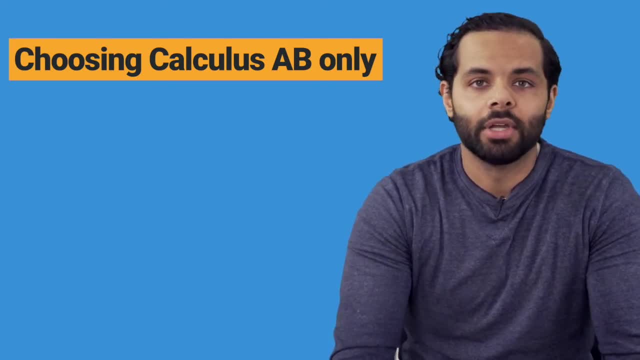 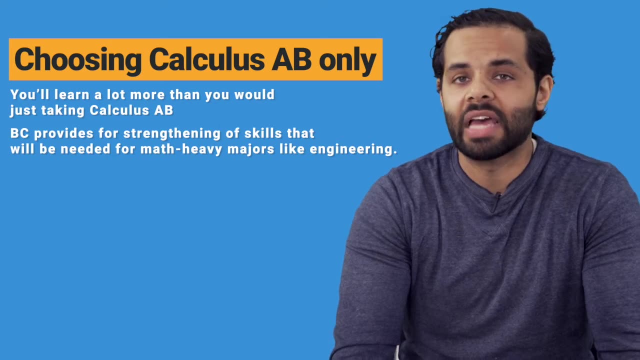 skipping Calc AB and taking BC might be your best bet. You'll learn a lot more than you would just taking Calc AB. BC provides for strengthening of skills that will be needed for math-heavy majors like engineering. It's possible to get credit for Calc 1. 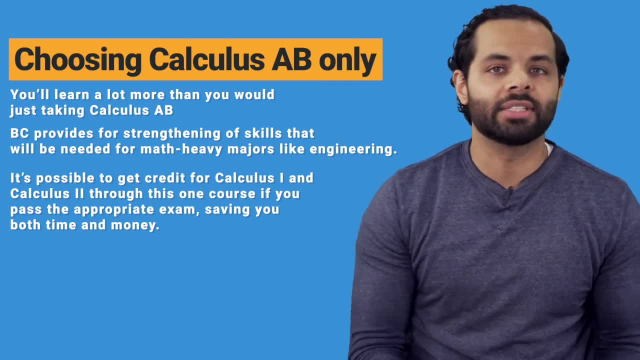 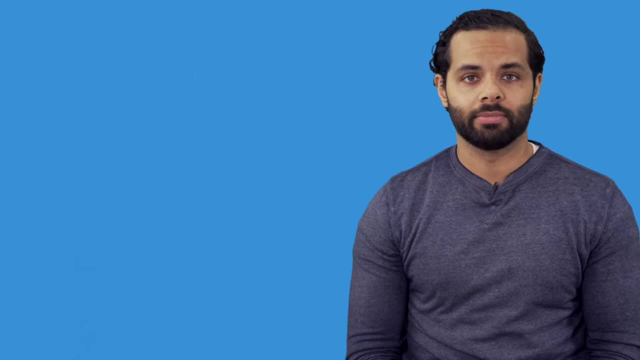 and Calc 2 through this one course if you pass the appropriate exam, saving you both time and money. Calc BC is viewed as a more challenging course, making it a better look on your transcript. Now let's move on to taking both Calc AB and BC courses. 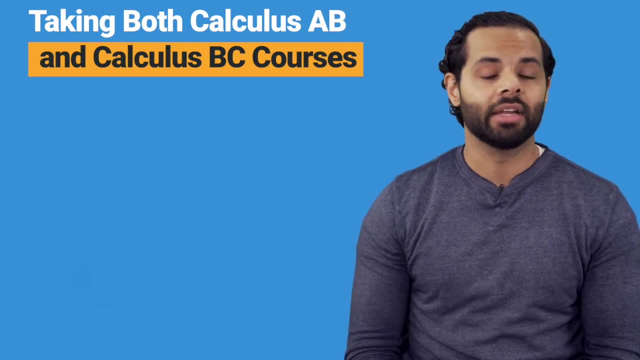 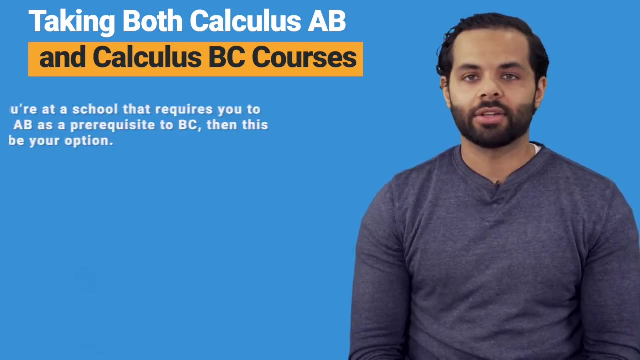 Most colleges will not give you credit for both Calc, AB and BC, so taking both courses would be pointless. However, some unique circumstances would make this a smart choice If you're at a school that requires you to take AB as a prerequisite to BC. 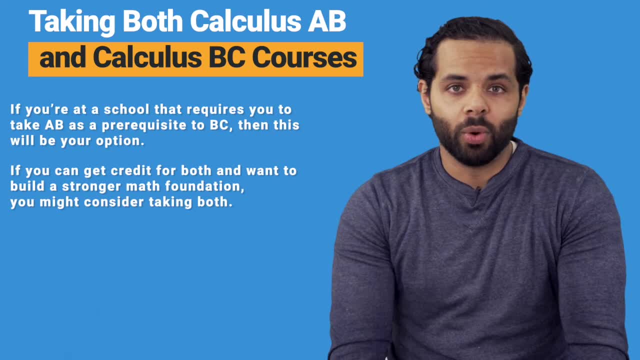 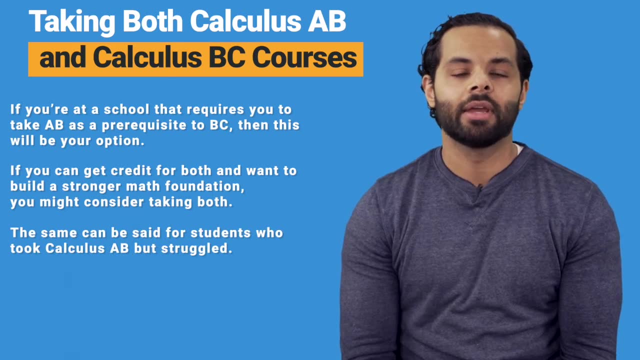 then this will be your option. If you can take credit for both and want to build a stronger math foundation, you might consider taking both. That makes sense. The same can be said for students who take Calc AB but struggled. Taking Calc BC can be a refresher course in a sense. 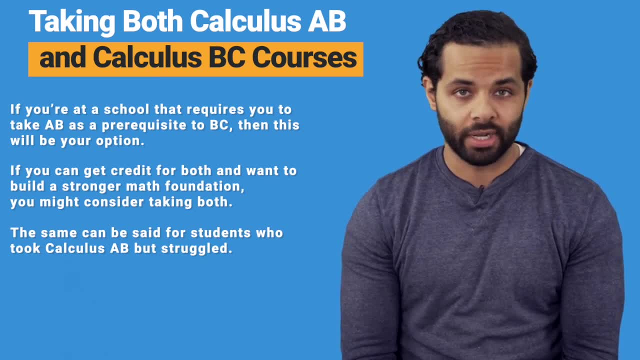 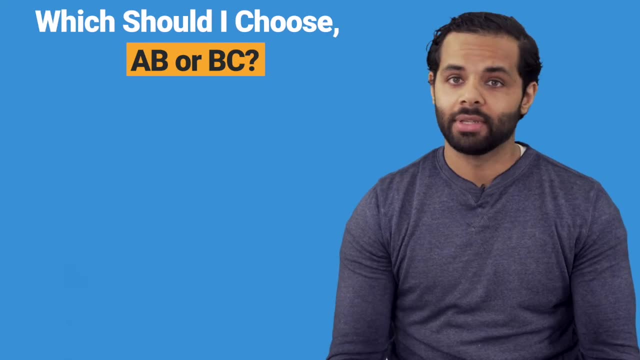 Just remember that Calc BC is a year-long course of study, so you wouldn't want to try and take both of these courses at the same time. Now, which one should you choose: Calc AB or Calc BC? Now you're at a crossroads where you must decide which course to choose. 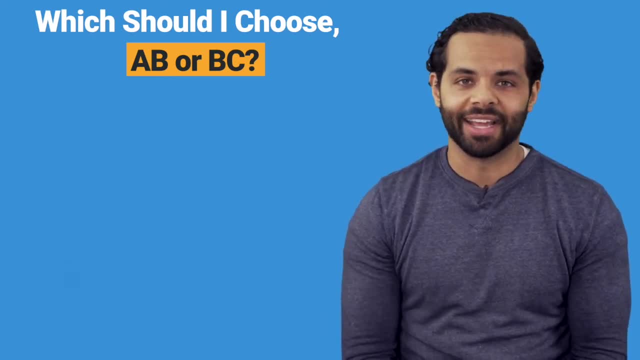 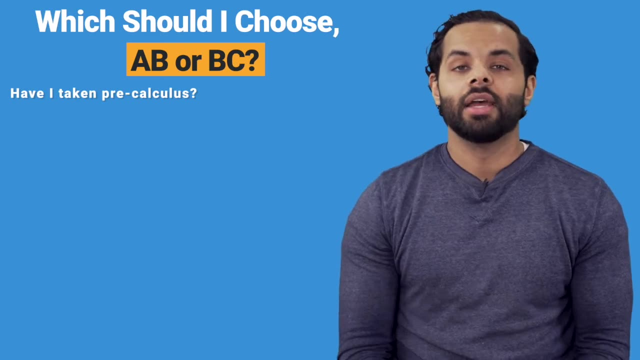 If you're still watching this video, then you might not have your answer yet. If so, ask yourself the following questions: Have you taken pre-Calc? Then consider AB and BC. Is there a placement exam at your school? Consider both Calc, AB and BC. 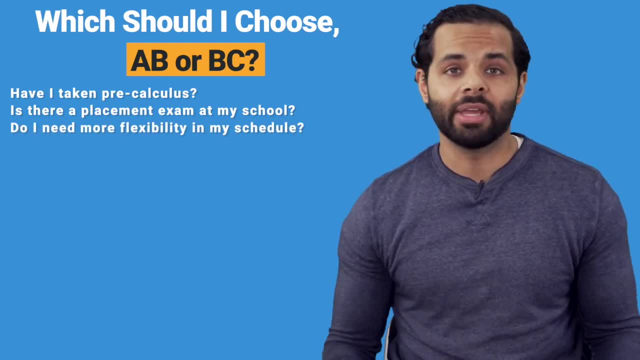 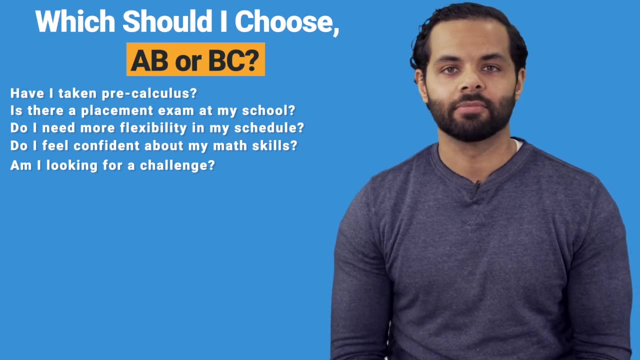 Do you need more flexibility in your schedule? Consider AB. Do you feel more confident about your math skills? Consider BC. Are you looking for a challenge? Consider BC. Are you worried that you might not do well on a fast-paced course? Consider AB. 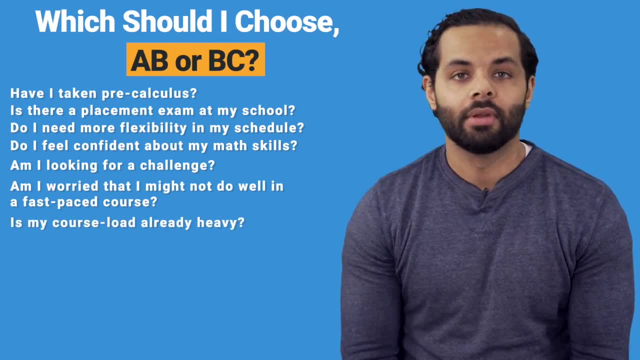 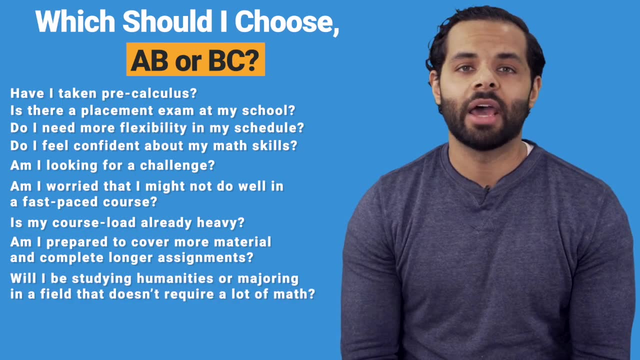 Is your course load already heavy? Consider AB: Are you prepared to cover more material and complete longer assignments? Consider BC: Will I be studying humanities or majoring in a field that doesn't require a lot of math? Consider AB: Will my future courses be math-heavy? 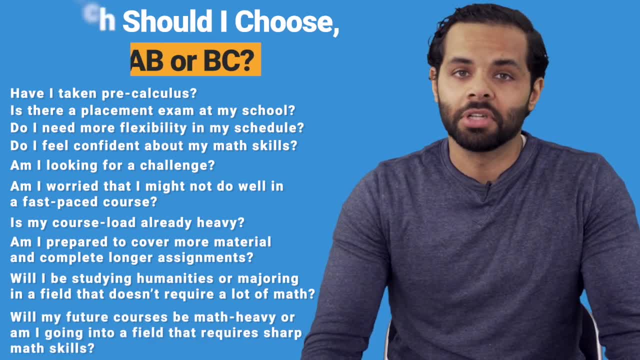 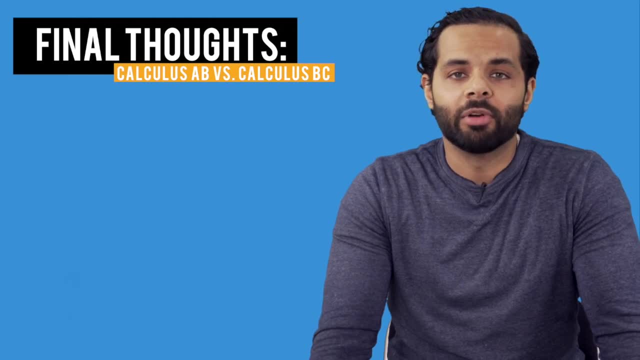 or am I going into a field that requires sharp math skills? Consider BC. When taking Calc AB, you will be learning about limits, definite integrals, derivatives, as well as a fundamental theorem of calculus. Calc BC will take your learning further, throwing in more advanced concepts.